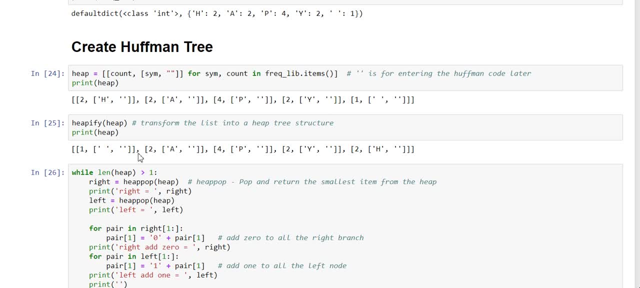 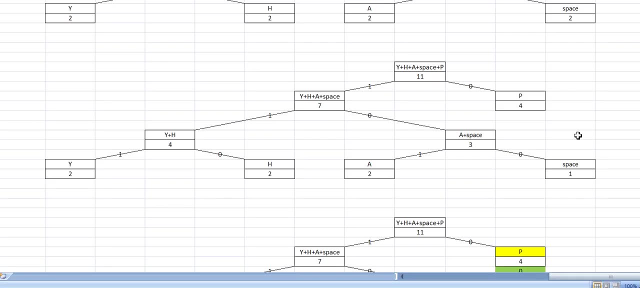 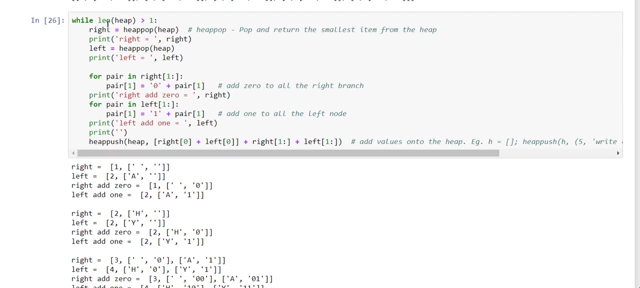 that for all the letters in the text And then you heapify it, which essentially means you transform the list into a heap tree structure which looks something like this, as I showed in the previous video, And then you loop through each item in the heap and you assign from the smallest item to the biggest item and you assign to the right or the left. 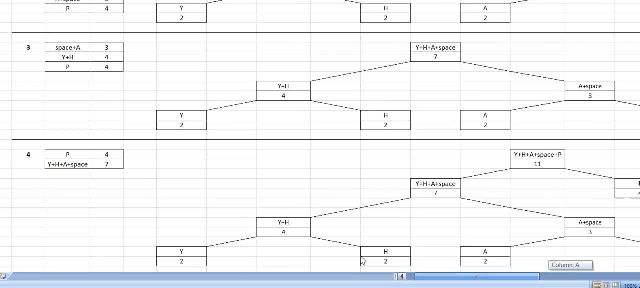 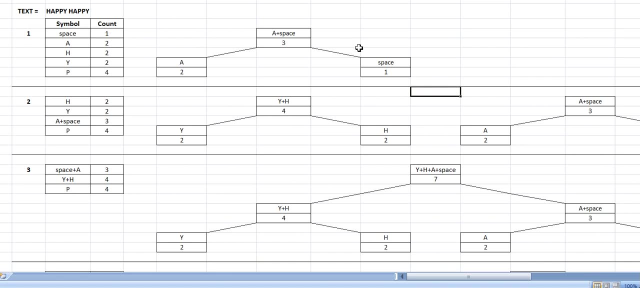 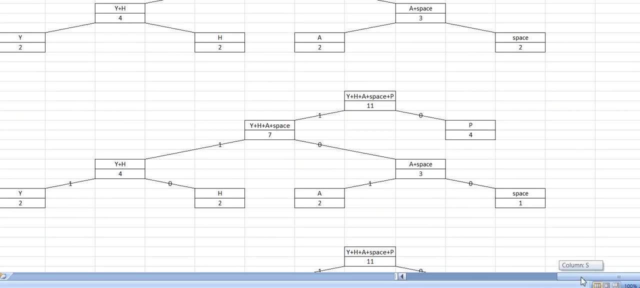 If you remember from the previous video I showed you a table of lists. You rank them and you start from the smallest item and assign to the left or the right to build the Huffman tree. so the first item is space on the right and a from the left, if you use the code. 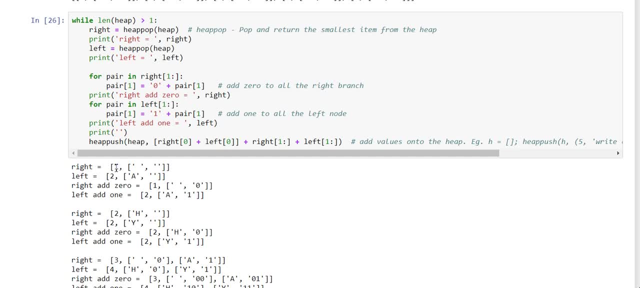 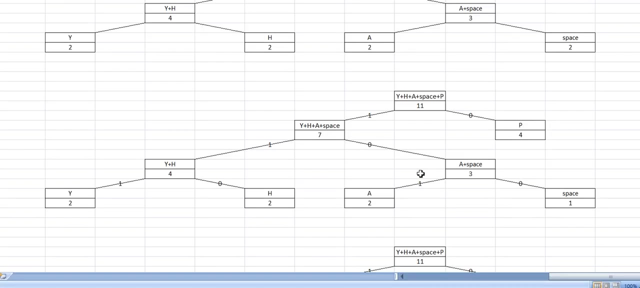 here you will see that if you print that you have a space on the right, a on the left, like space on the right, a on the left, and they will assign 0 to the right branch and 1 to the left branch, 0 to the right, 1 to the left. after you do it, you 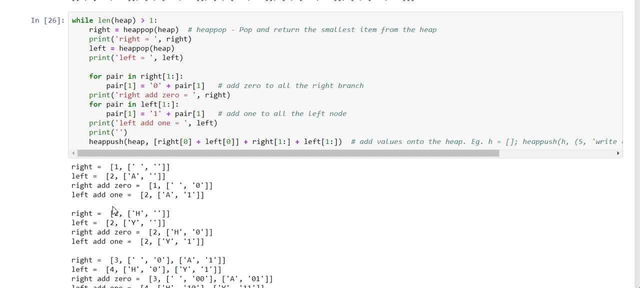 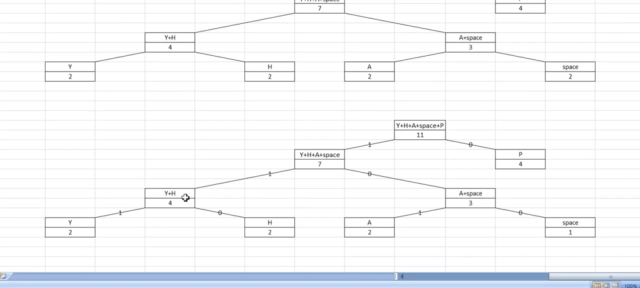 go look. in the second loop you look for the second smallest item, which you have- h and y, h and y here, and in the third loop you have space a, h and y, space a, h and y and you just repeat the loop until you get the top, and then you 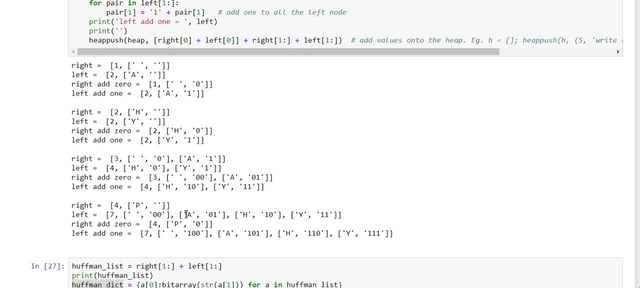 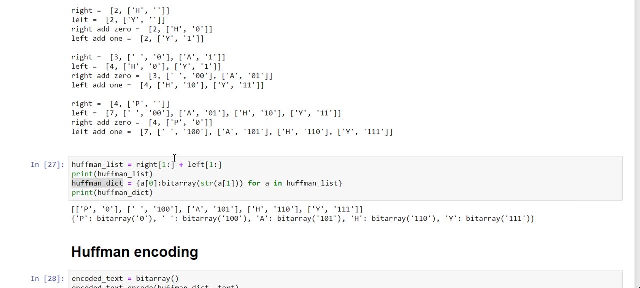 have your half man codes. there's a sign to the right or the left branch and you retrieve them by correcting all the lists. within the list of this, of the right and left, you ignore the first item, because the first item is the card you are not interested in. if you print it, it should look something like this: you have